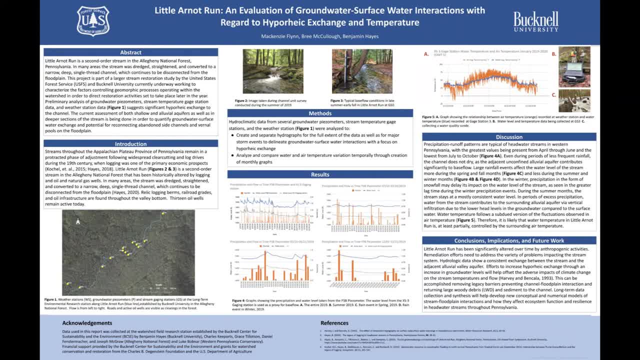 As seen in Figure 5,, water temperature follows the subdued version of the fluctuations observed in air temperature, indicating that the water temperature in Litter-Arnott Run is partially controlled by the surrounding air temperature. Little Arnott Run has been significantly altered over time and remediation efforts need to address this. 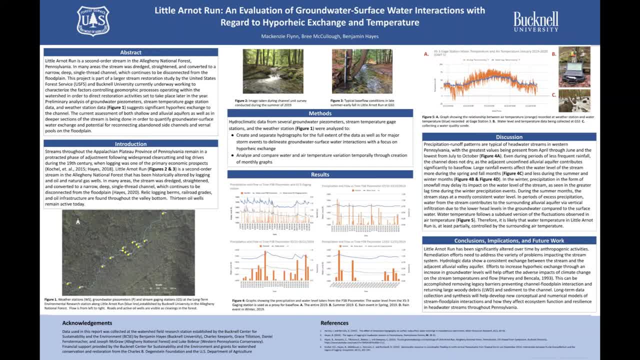 We believe that efforts to increase hypereic exchange through an increase of groundwater level will help offset adverse impacts, along with remediation efforts, including reconnecting the floodplain and building large woody debris structures. Thank you for your time. 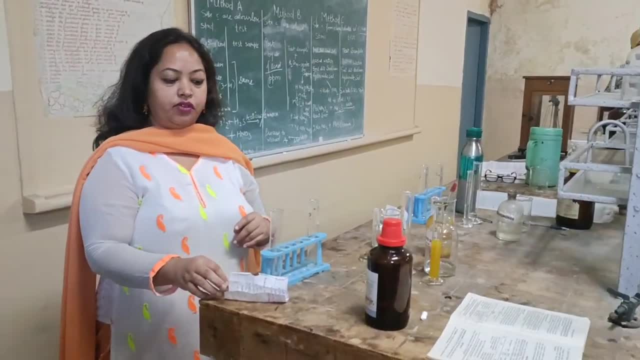 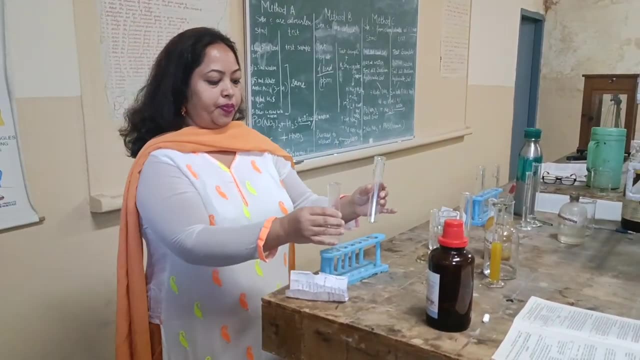 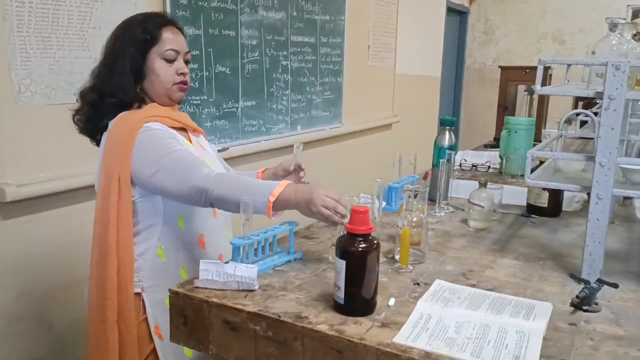 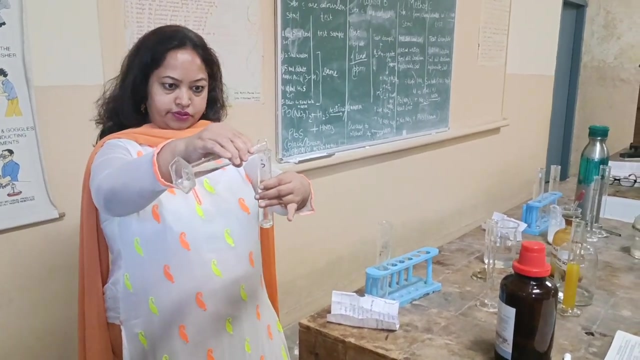 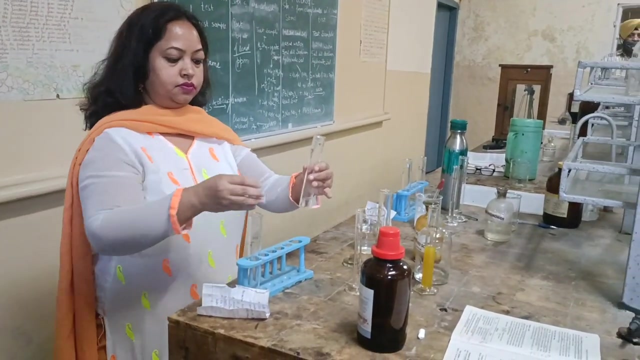 We are going to start the method A for heavy metals, for which we have taken two Nestle cylinders. One is standard, another is test. So in the standard we will add 2 ml of lead standard solution, 5 ml ammonia to adjust the pH up to 3 to 4.. And in the test sample: 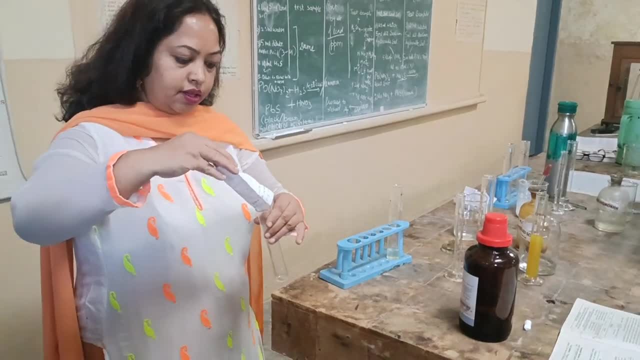 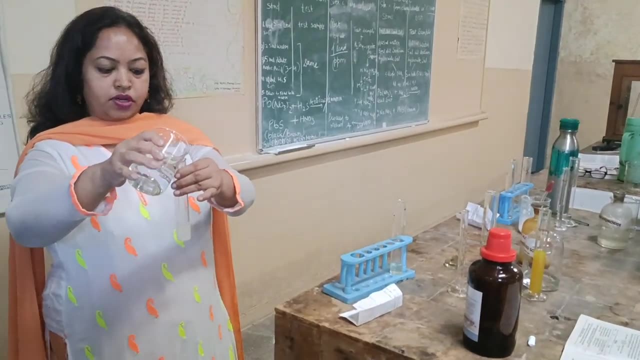 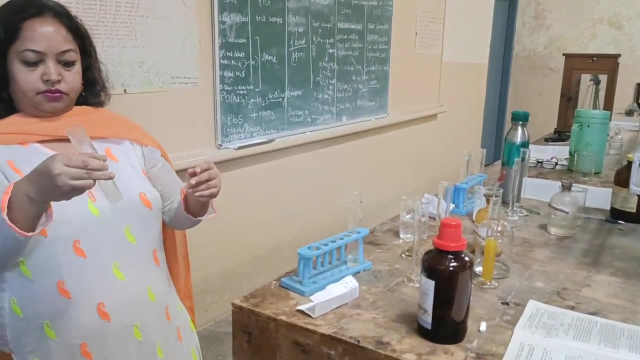 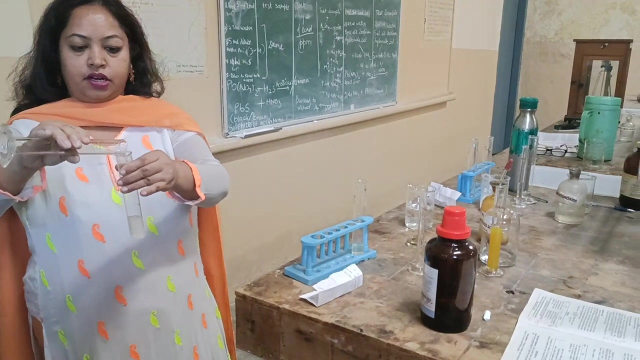 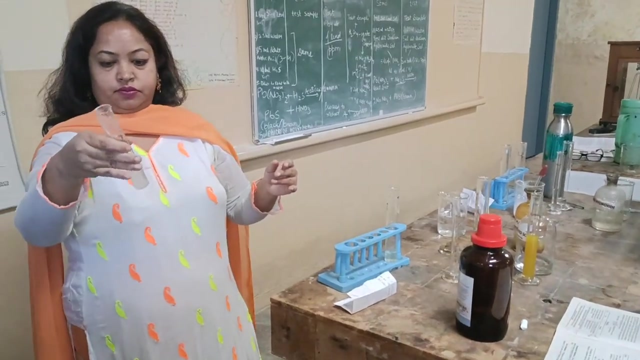 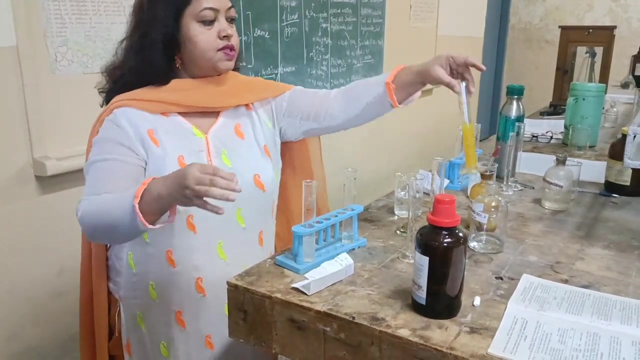 we have taken sodium chloride in which we have to analyze the limitase for heavy metals. We will dilute it with water, We will dissolve the sodium chloride And then we will add 5 ml of ammonia again in the test to adjust the pH, And in both standard and test we are going to add 2 ml of lead.